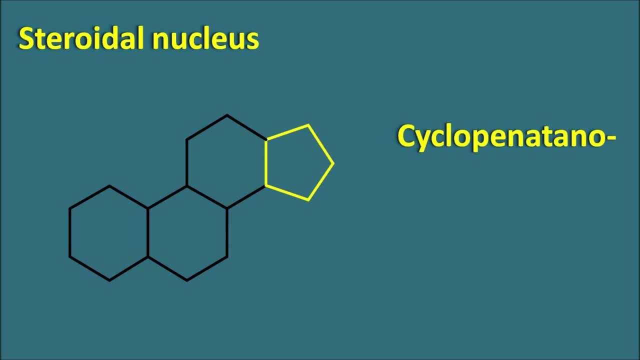 So this five member ring system is nothing but the cyclopentane. so we can call it a cyclopentano because it is going to be fused, and it is going to be fused with a phenanthrene like nucleus, but which is saturated completely, so we can call this as perhydro phenanthrene. 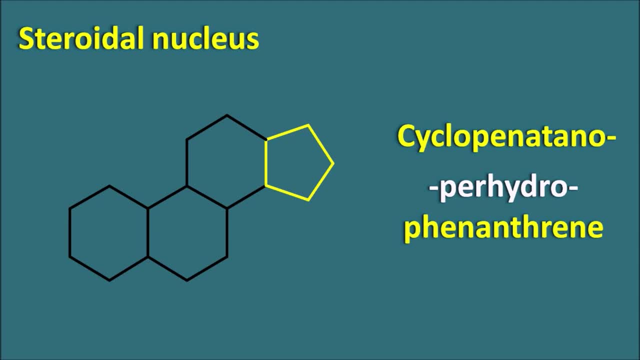 So steroid nucleus can be called as a cyclopentano perhydro phenanthrene nucleus, because it is obtained from the fusion of the cyclopentane ring as well as the perhydro phenanthrene ring. Now let us see the numbering of the steroidal ring systems. First, we have to 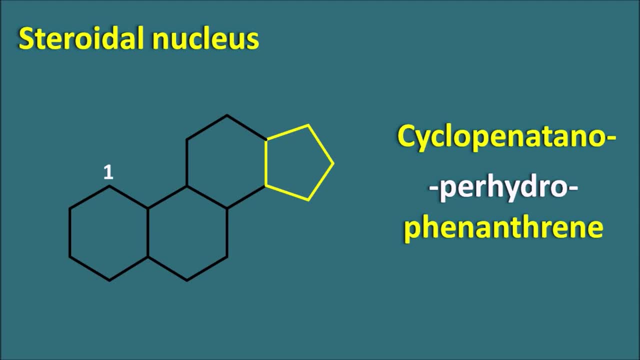 start the numbering from here and we can continue the numbering to the two rings which are present in the horizontal lane. So this is one, two, three, four. in the polycyclic ring systems we are not giving the numbering to the bridge heads or fusion atoms, but here we are giving the numbering to the bridge head, so this is five. 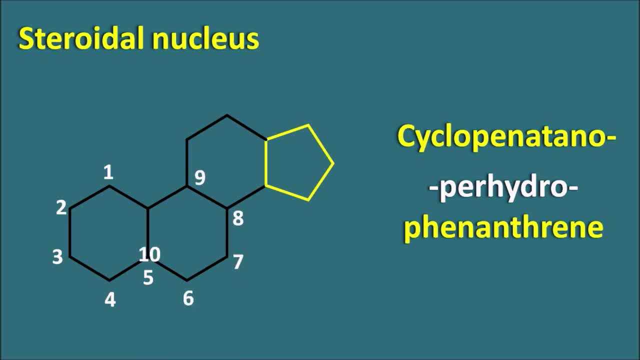 six, seven, eight, nine, ten. In this way we have completed the numbering to these two rings which are horizontally fused. Now let us go with the next ring. this is eleven, twelve, thirteen, but we are going to give the numbering in a shape, so this is thirteen. 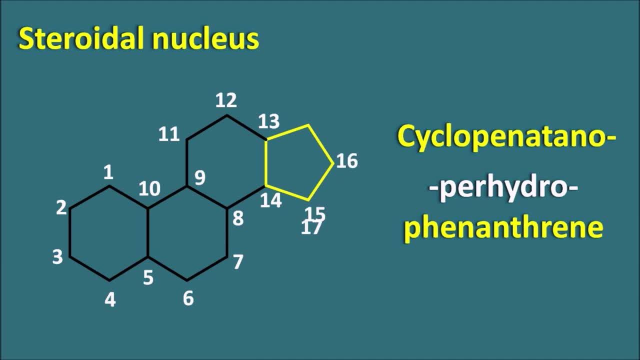 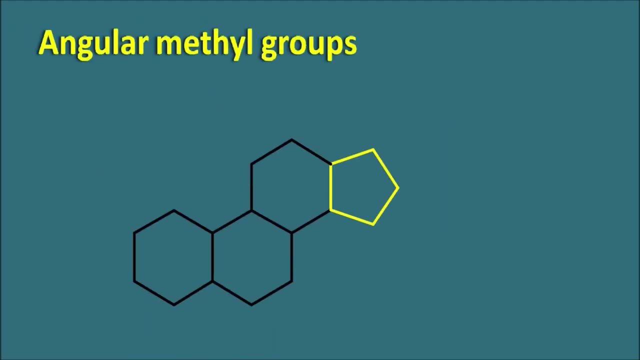 and this is fourteen, fifteen, sixteen and seventeen. So this is the numbering to this steroidal ring system. Now this basic steroidal nucleus is having the seventeen carbons. so this is a C 17 steroidal nucleus. Now let us see the angular methyl groups To this steroidal nucleus. 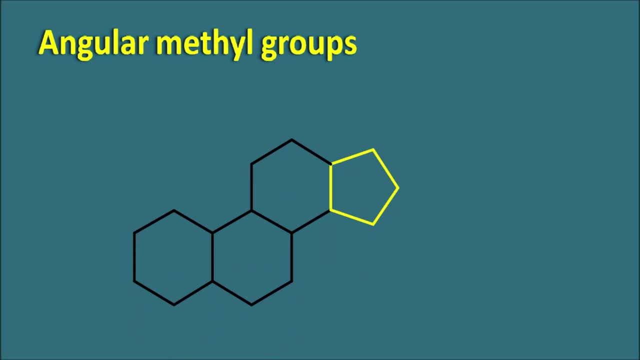 we can add the methyl groups at the angular positions to increase the chain length. For example, one of the methyl group can be attached here and this methyl group can be numbered as 18 carbon, And another methyl group can be attached here. this is the 19th carbon. 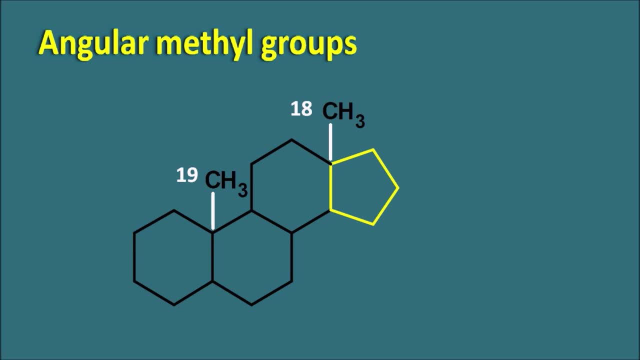 So here we are, coming from the upward to the downward. so one of the methyl group attached at the cyclopentano ring is the 18 and other methyl group is the 19.. Now let us the side chain at the 17th position. Let us see how we can give the numbering in the steroidal nucleus, if it is. 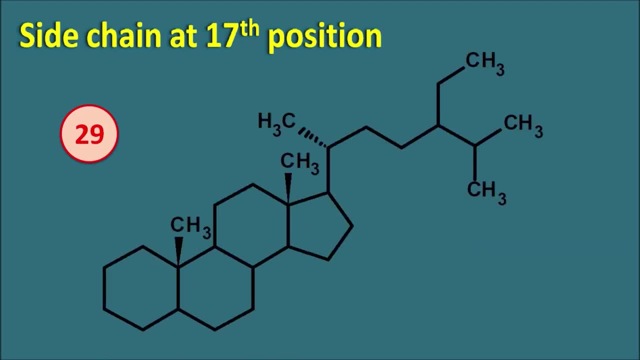 having the 29 carbons. So this is the structure of a steroid having the 29 carbons, and all we have is the numbering of the 20th. carbon and angular methyl groups are given the numbering 18 and 19. Then we can continue the numbering from 20 to the side chain, so this is the 20.. After that we have 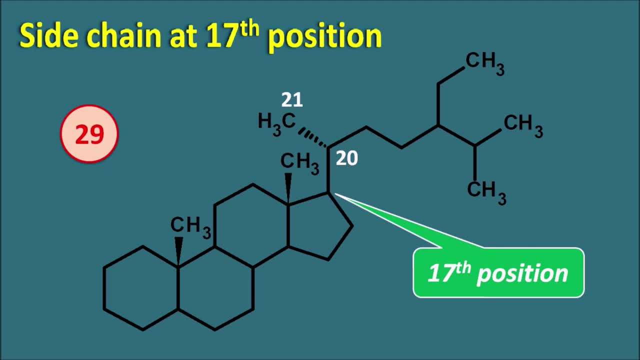 to give the numbering 21 to this carbon, and this carbon is attached by the alpha portion to the side chain. then we can continue: 22, 23, 24, 25 and here 26 and 27.. In this way we can continue the numbering in the side chain up to the 27 carbons, Then the remaining carbons which are attached at 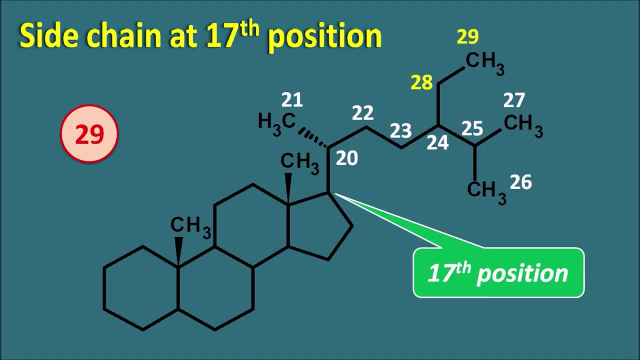 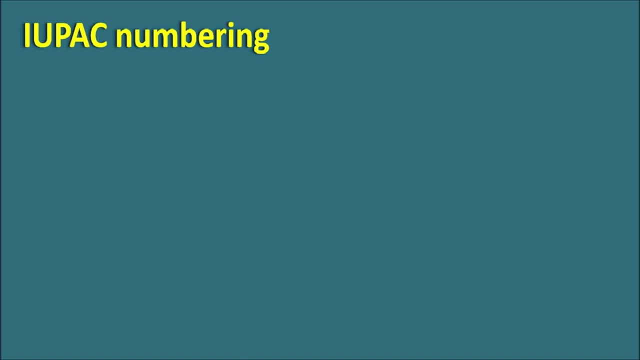 the 24 position can be numbered as 28 and 29.. So this is the numbering system for the steroids having the 29 carbons. But according to the IUPAC there is a little changing in this numbering system. For example, if you consider the 29 carbon steroidal nucleus, so this is a 29 carbon steroidal. 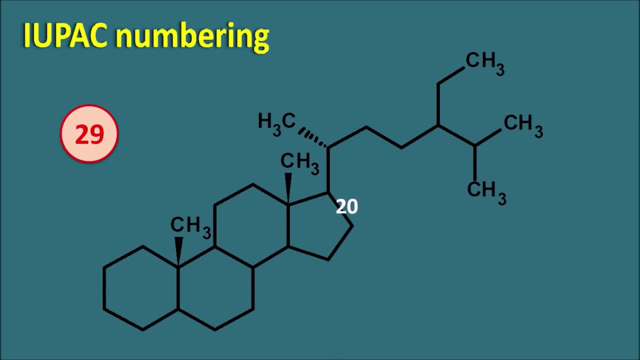 ring Now. already we have seen we have given the numbering to the side chain like 20, 21, 22, 23, 24, 25. whatever the numbering we have given to the 28 and 29 are not considered in the IUPAC and 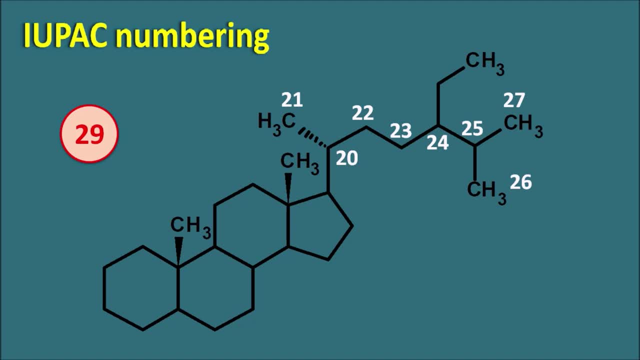 they are considered as a side chains attached to the 24th portion and they are denoted as 24: 1 and 24: 2.. So, according to the IUPAC, we are giving the numbering up to the 27 only, and the other two carbons can be represented as 24: 1 and 24: 2.. 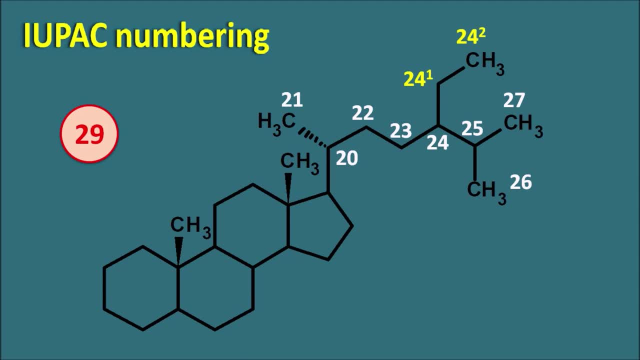 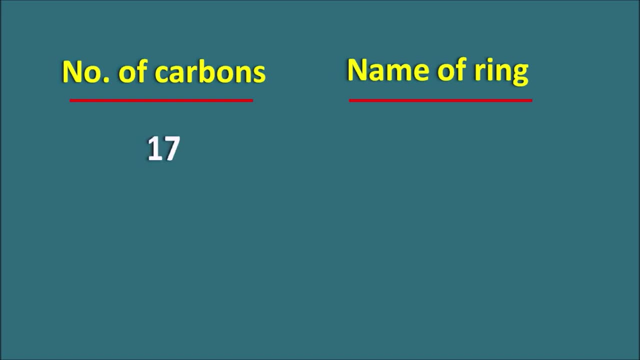 So this is a little change according to the IUPAC numbering. Now let us see the. what are the number of carbons and what is the name of the ring system. So the basic ring system is hanging the 17 carbons and that ring can be called as gonan and 18 carbons it can be called as e strain 19. 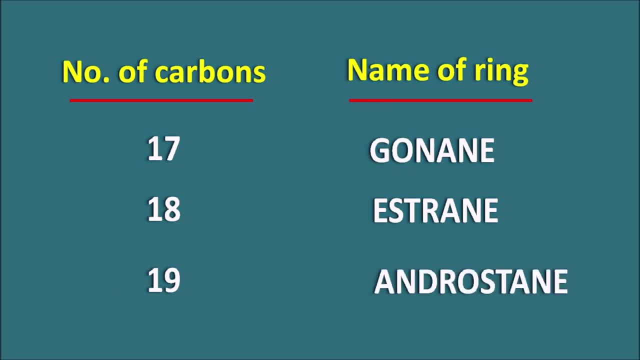 carbon. it can be called as androstene. you can see that these nucleus are going to differ by one: 17, 18, 19.. so you can easily remember it is a gonan e strain and androstene. then after the 19, we are: 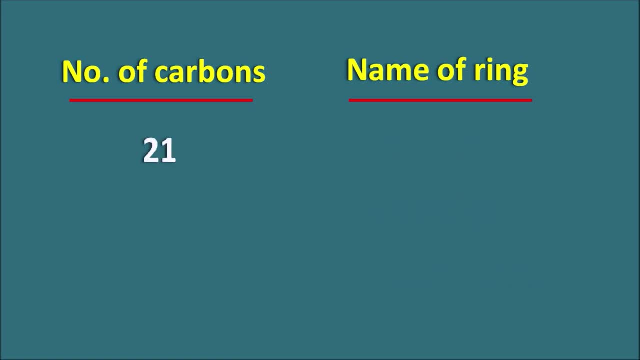 not going to the 20, we are jumping to the 21. 21 is the pregnant, then 24, we are again jumping to the 24, that is, colon 27, colistin. and here you can see, these are going to differ by three. the previous one they are going to differ by one, and here they are going to differ by three: 21, 24, 27. 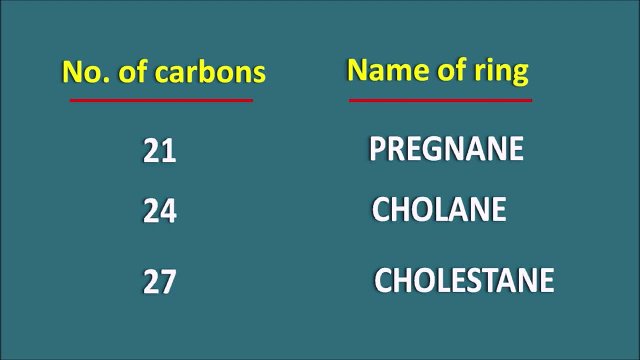 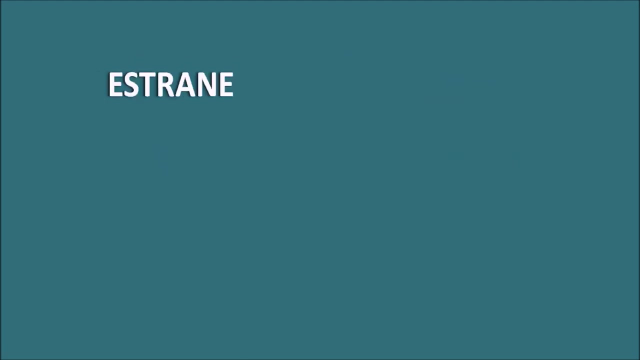 which are the pregnant colon colistin, pcc, pregnant colon colistin- then we can have, if you have the steroids which are not present in the humans but they can be present in the animals and plants. so 28 is the ergo stain and 29 is the stigma sting in this. 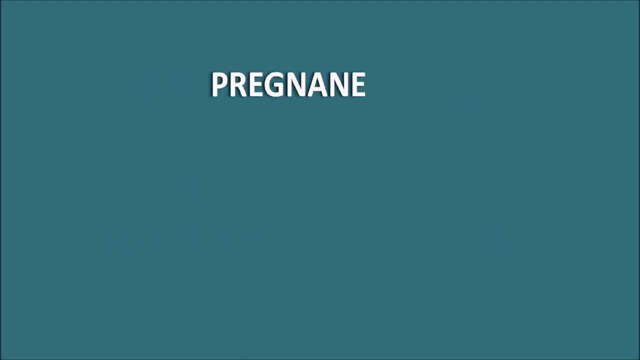 like the testosterone. Similarly, pregnen nucleus is present in the progesterones as well as is also present in the corticosteroids. These corticosteroids are of two types: glucocorticoids as well as mineralocorticoids. Similarly. 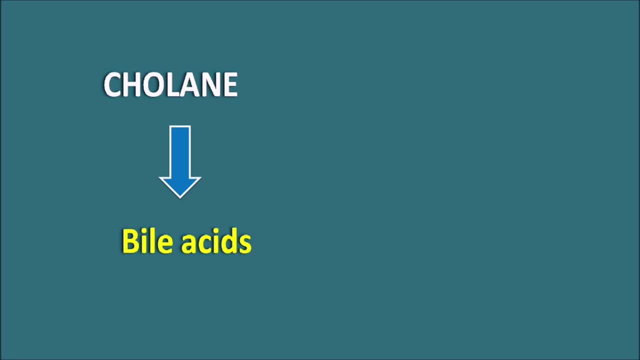 another nucleus: choline is present in the bile acids and colistin is present in the cholesterol. Ergostin is present in the ergosterol and stigmastin is present in the stigmasterol. In this way, different types of steroidal. 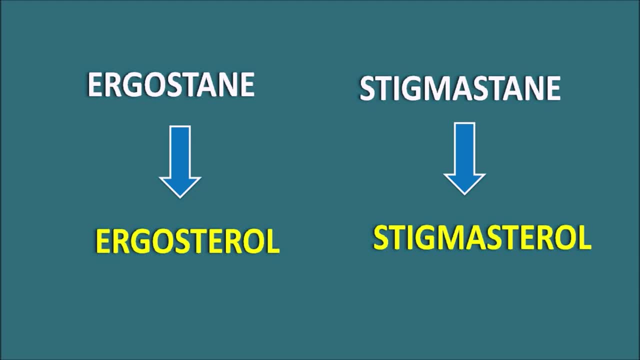 nucleus are present in the different types of steroidal compounds. So now let us see the different types of steroidal nucleus and how they are going to be modified to produce the different types of steroidal compounds. First is the C 17 steroids. We have already seen this is a basic nucleus of the 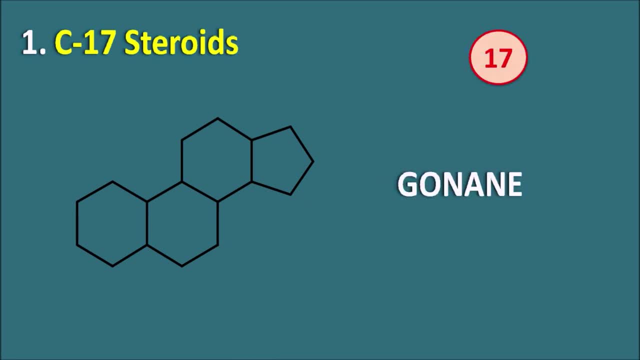 sterol ring which is in the 17 carbons. This nucleus is called as gonan, but there is no compound is present with the gonan nucleus and it can be modified to produce the E strains as well as the progesterones. Second one is the 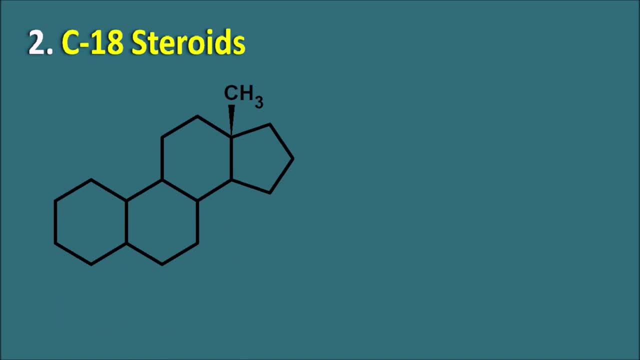 C 18 steroids, So C 18, are having the basic nucleus like this. and here you can observe, because of the one angular methyl group, these are having the 18 carbons and this nucleus is called as E-strain. This E-strain is: 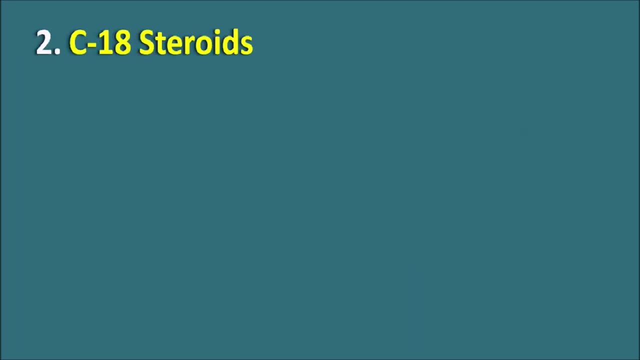 present in the various types of estrogens. So let us see the first structure of the estrogen. this is the E-stron. In this E-stron you can see that the E-strain nucleus is somewhat modified, such that the first ring is converted into an aromatic ring. You can observe the three double 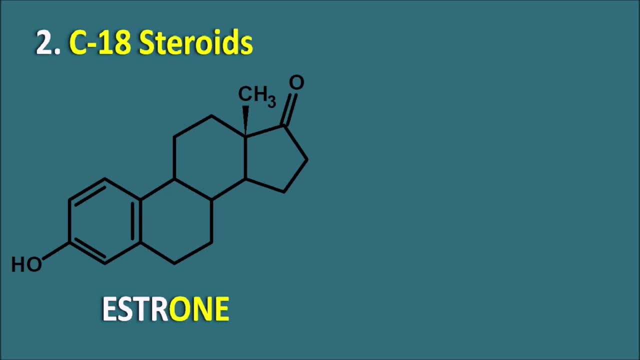 bonds are present and because of presence of three double bonds within a single cycle. now this ring system becomes aromatic in nature and apart from this aromatization, it is also having a OH group at the third position and a ketone group at the 17th position. This ketone group is: 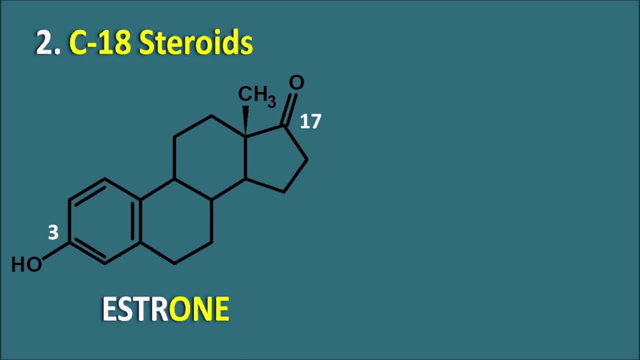 going to be identified with the suffix on within the name. So E-stron indicates having a ketone at the 17th position. Similarly, another estrogen is the E-stradial. In the E-stradial again, we can observe a OH group at the third position, 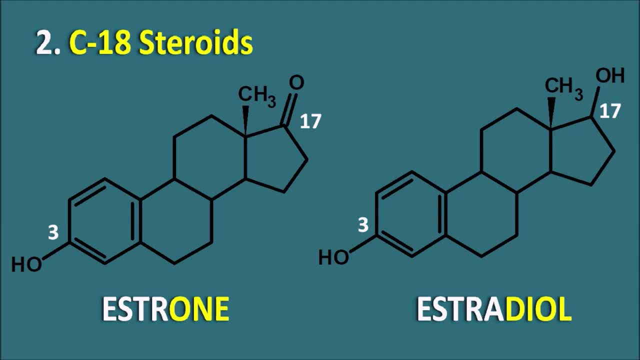 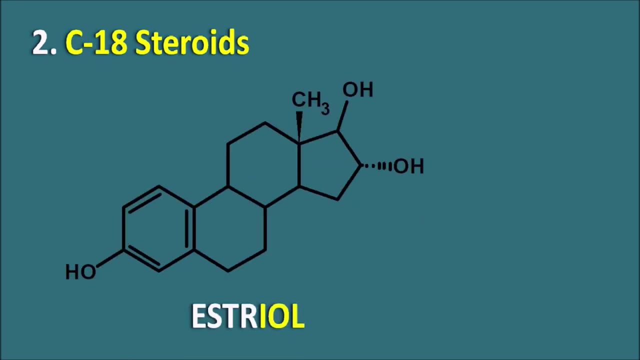 But at the 17th position, instead of the ketone group it is converted to alcohol group, So E-stradial, it is having the two hydroxyl groups, that is a dial group, So, which is at the third position as well as the 17th position. Another estrogen is the E-strial. Now in the E-strial, the OH groups. 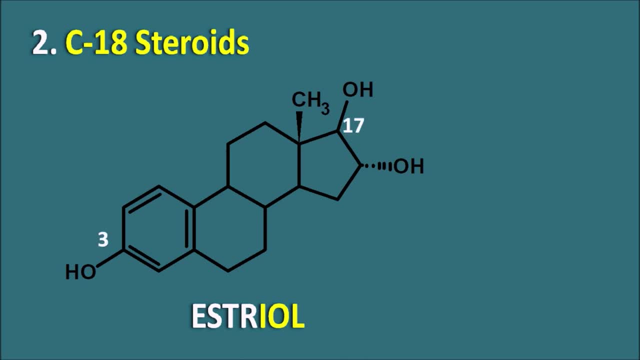 are present at the third position as well as at the 17th position, and apart from these two OH groups, an extra OH group is present at the 16th position which is attached by alpha linkage. So a 16 alpha hydroxyl group is present along with the dihydroxy groups. So totally it is having 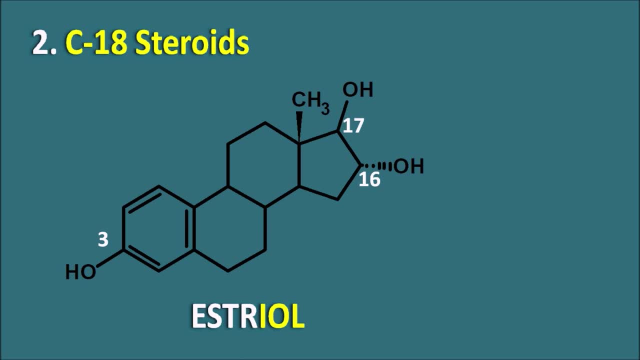 the three hydroxyl groups. that's why it is called as E-strial. E-strial is having the three hydroxyl groups at the third, 16th and 17th positions. So these are the three estrogens which are derived. 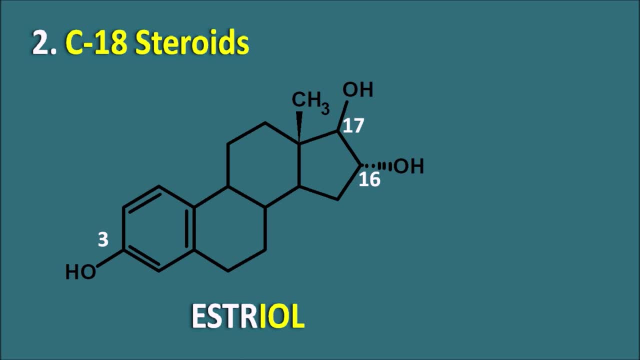 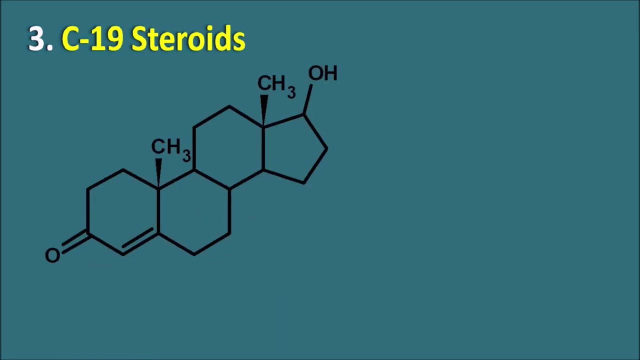 from the E-strain nucleus, But this E-strain nucleus is going to be modified such that the first ring is going to be aromatized by introduction of three double bonds. Third type of steroids are C-19 steroids and this is one of the C-19 steroids and you can observe it is having the 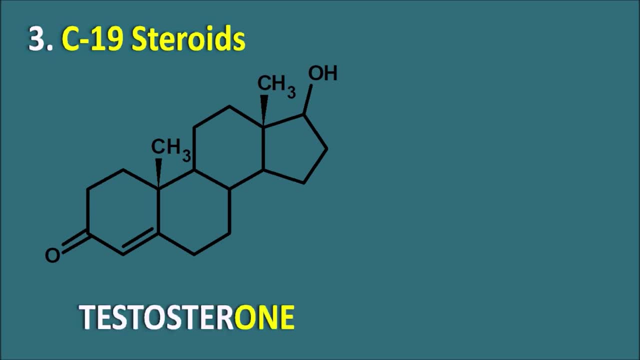 androstene nucleus and one of these hormone is the testosterone. Again, here this androstene nucleus is going to be modified at the different positions. Third position, it is having a ketone group, Fourth position, it is having a double bond and 17th position, it is having a alcohol group. 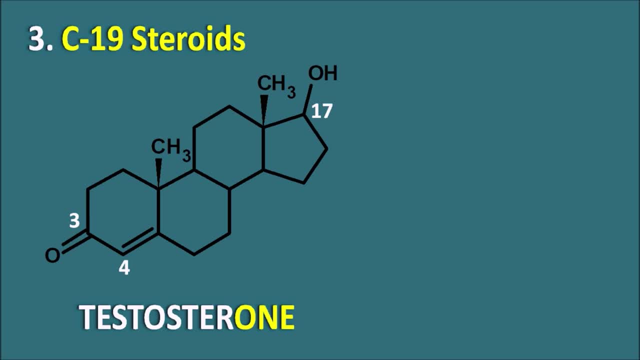 So testosterone is coming from the androstene, but this androstene is having a double bond at the fourth position, so it can be called as androstene. So testosterone can be written as androst-4-ene, because double bond is present at the fourth position. Androst-4-ene- 17-beta-ol. 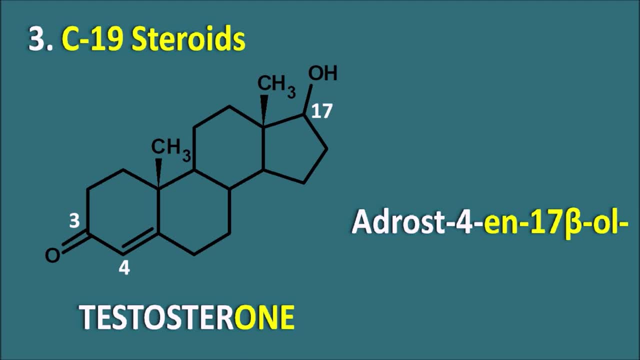 The 17th position, hydroxyl group, is attached by beta linkage, so 17-beta-ol. and third position, ketone group is there, so which can be denoted as 3-ol, So testosterone is the androst-4-ene 17-beta-ol 3-ol. 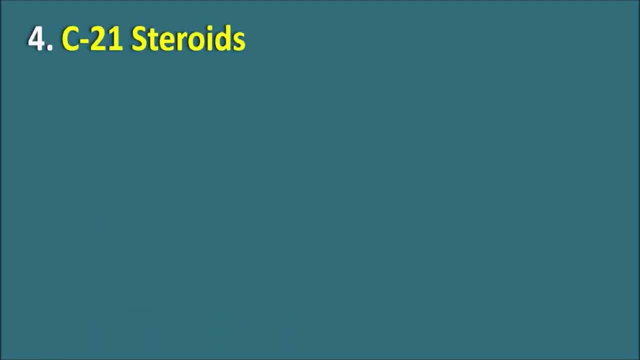 That is the testosterone. And fourth type of steroids are the C-21 steroids. So this is one of the C-21 steroids and they are having the pygmy nucleus, and here one of the hormone is the progesterone, And here you can observe that it is having the 21 carbons. 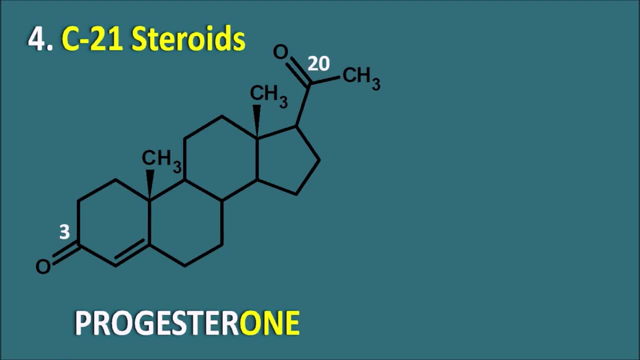 and at the third position it is having a ketone group as well as 20th position and their ketone group, So it is having a 3-20-dione. and fourth position, just like the testosterone, it is also having a double bond. So progesterone is nothing but the. 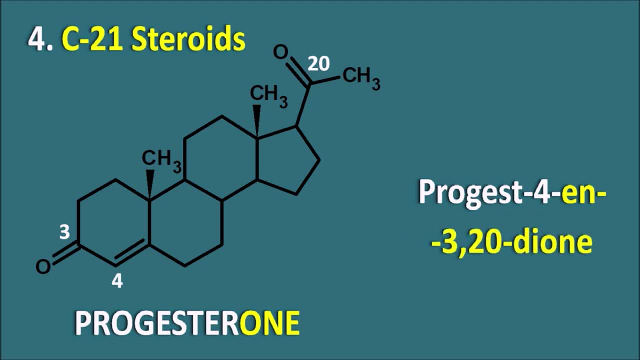 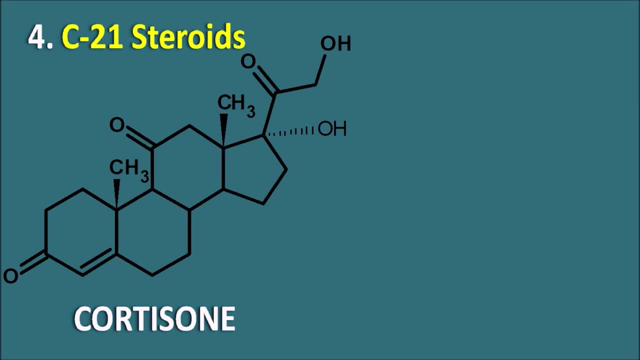 progesterone-4-ene, 3-20-dione, Similarly corticosteroids. one of the corticosteroids is the cortisone. In this cortisone we can observe the ketone groups at the third position, 11th. 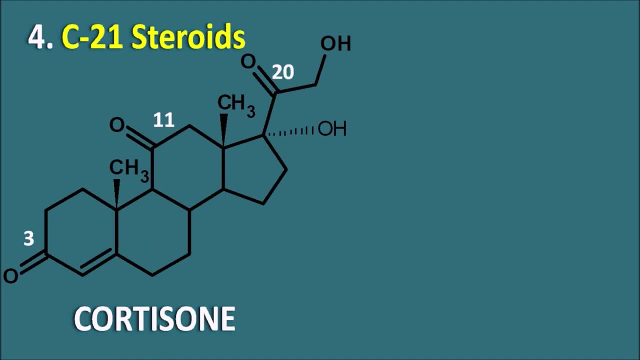 position as well as the 20th position. So, just like the progesterone, it is also having the ketone groups at the third and 20th position, but apart from this, it is also having a ketone group at the 11th position And again it is having a fourth position, a double bond, just like the. 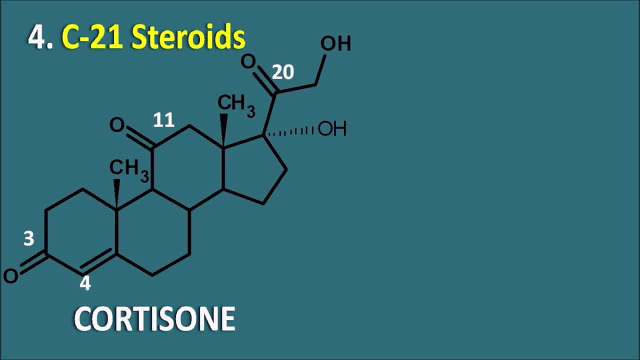 progesterone, But apart from this, it is also having a ketone group at the 11th position, but apart from this, it is having a hydroxyl group at the 17th position, which is attached by alpha linkage, and another hydroxyl group at the 21st position within the side chain. 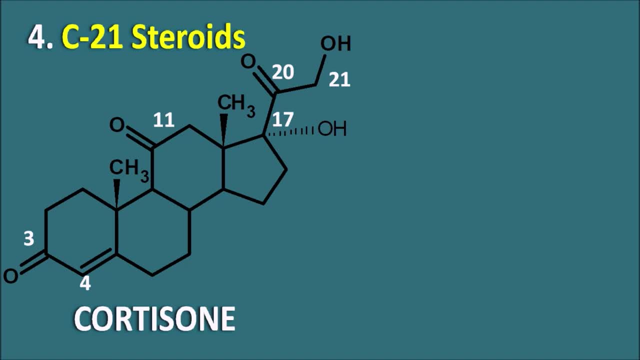 in this way, cartosone is having the three ketone groups at the third, 11 and 20th positions and two hydroxyl groups at the 17th and 21 positions. similarly, another corticosteroid is a hydrocortisone in the hydrocortisone because the prefix hydro indicates one of the ketone group. 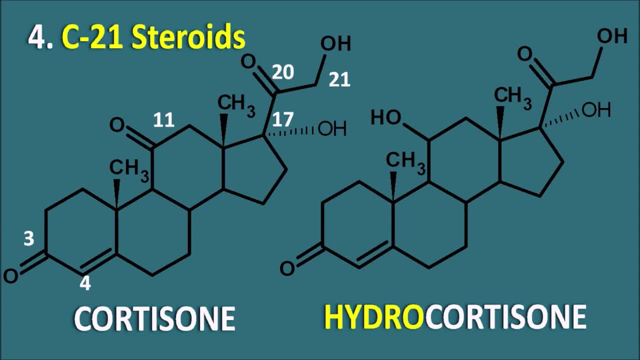 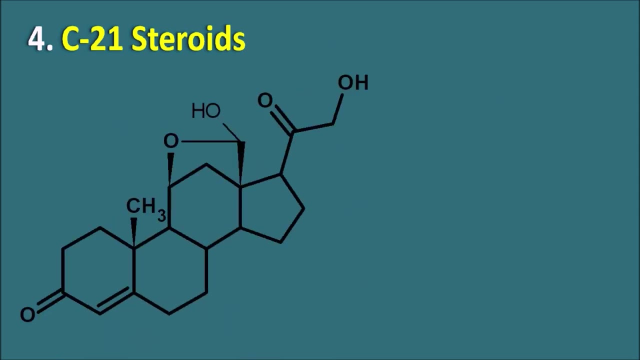 is converted into a hydroxyl group. you can observe here, at the 11th portion, ketone group is coming to hydroxyl group. so hydrocortisone is a reduced form of the cartosone, where the ketone group at the 11th position is converted into hydroxyl group. similarly, another one is the. 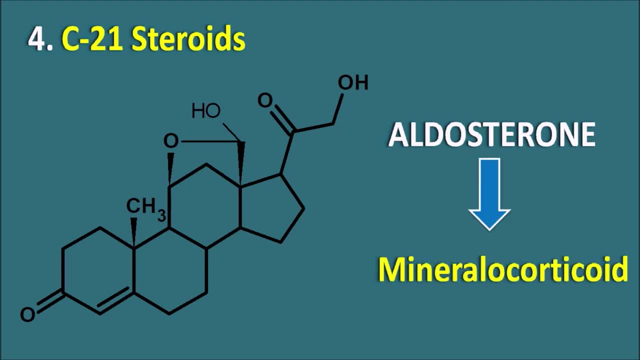 aldosterone. aldosterone is one of a mineralocorticoid. again, this aldosterone is having the prignan nucleus but if we compare with the glucocorticoids it is having a oh group at the level of the hydroxyl group and the hydroxyl group is the hydroxyl group and the aldosterone group is. 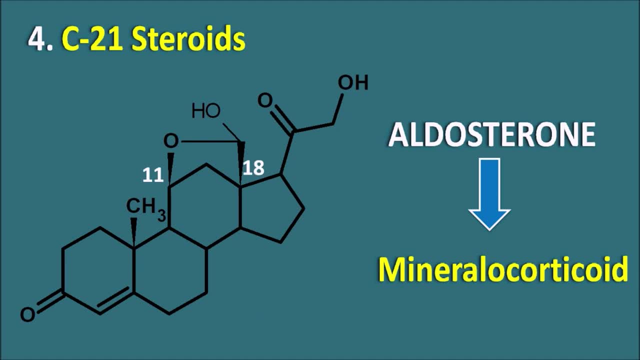 at the 11th position and an aldehyde group at the 18th position. this oh group and aldehyde groups can be combined to form a cyclic form, so aldosterone may be present as an open chain as well as in the closed form at the 11th and 18th positions. next one is a c24 steroids, so these are 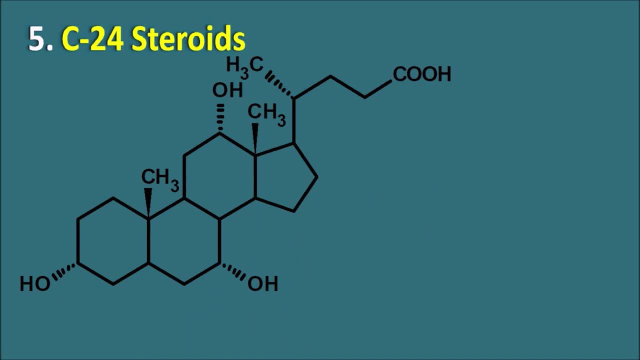 c's 24 steroid. you can see the side chain is somewhat increased and these are having the choline nucleus. so choline nucleus will give the bile acids. so one of the bile acid is the colic acid and you can easily observe the side chain is having the carboxylic acid. so it is the sdk nature. 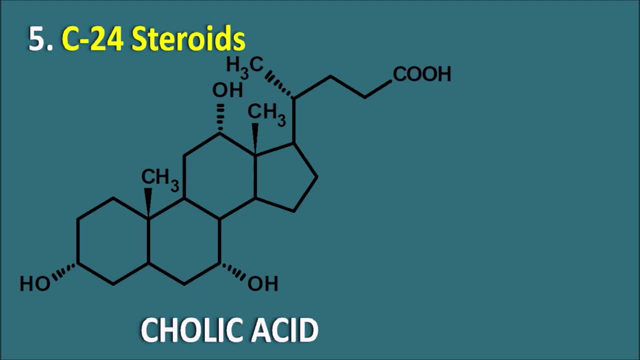 which is the identified by its suffix acid, and it is having the oh groups at the different positions, third position, seventh position and twelfth position. all these oh groups are attached by alpha linkage, so colic acid can be written as 3, 7, 12, trihydroxy choline, 24 oic acid, because the 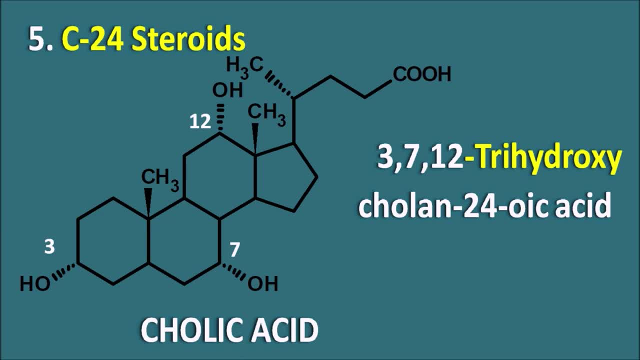 carboxylic acid is present at the terminal. that is the 24th position. so it is a choline 24 oic acid. and here we should not confuse this with the cholestane. cholestane is given the cholesterol, but choline is given the colic acids. this colic acid is: 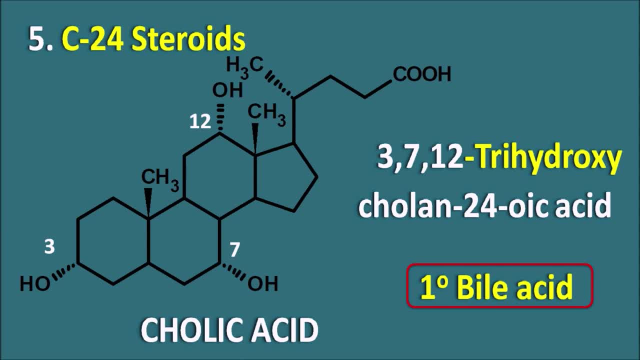 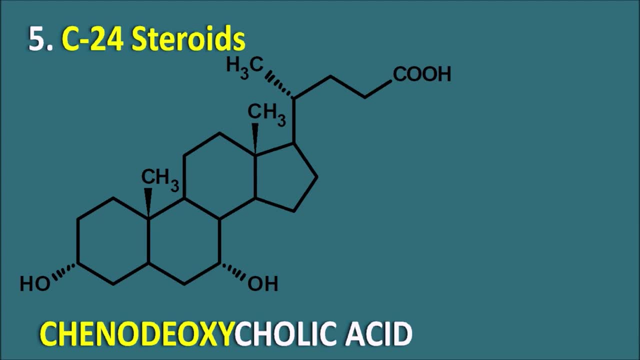 the primary bile acid, which is responsible for the sequestering of the fatty acids. similarly, another bile acid is the chino deoxy colic acid. this is having the oh group at the third position as well as the seventh position, but it is not having a oh group at the 12th position. 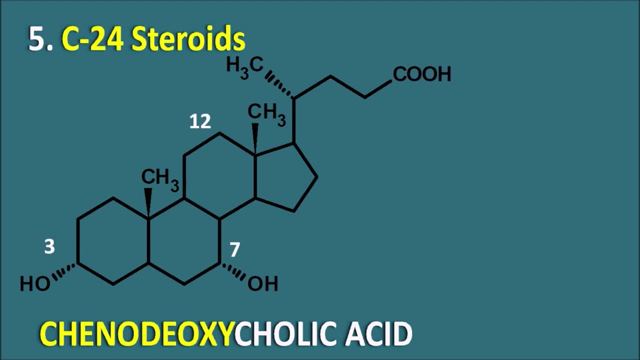 so it is having the hydroxyl groups only at the third and seventh positions. so that's why chino deoxy colic acid can be written as 3, 7 dihydroxy choline, 24 oic acid. again, chino deoxy colic acid is a. 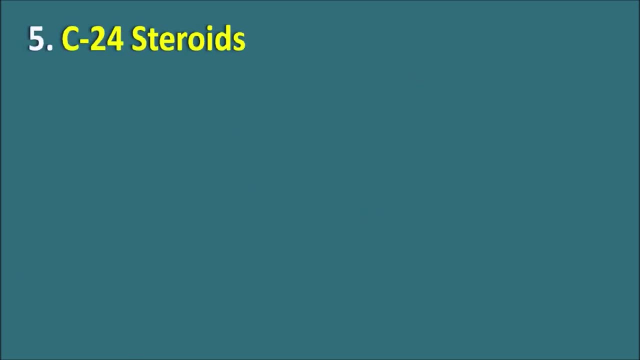 primary bile acid. from this primary bile acids now we can get the secondary bile acids, and this is one of the secondary bile acid. this is the deoxy colic acid. now this structure is having the oh groups at the third position as well as at the second position, so it is having the oh groups at 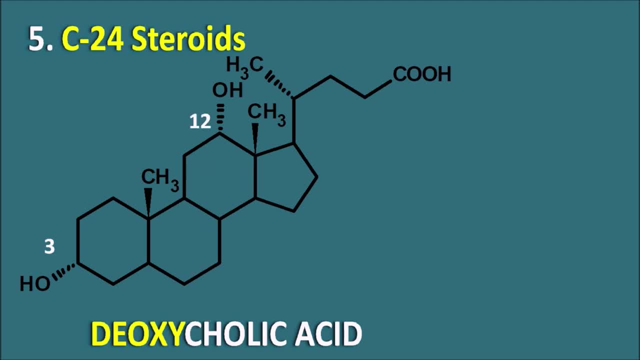 the 12th position but it is not having the oh group at the seventh position. so deoxy colic acid is the 312 dihydroxy choline 24 oic acid and this deoxy colic acid is obtained from the bile, obtained from the primary bile acids, so it is a secondary bile acid. similarly, another secondary bile acid is: 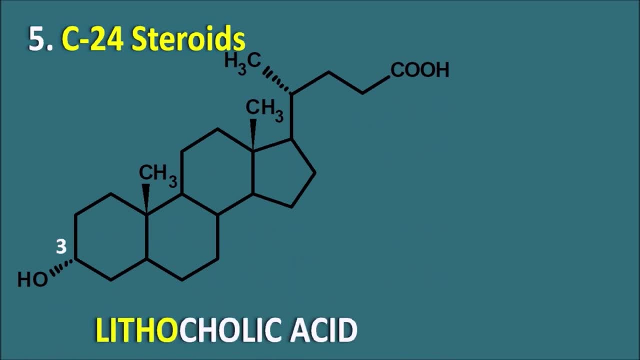 the litho colic acid. litho colic acid is having the oh group only at the third position and is the becausebile acide and since it is derived from the primary bile acids, it is a secondary bile acid. in this way, bile acids are having the c24 steroidal ring and their derivatives of the choline nucleus. 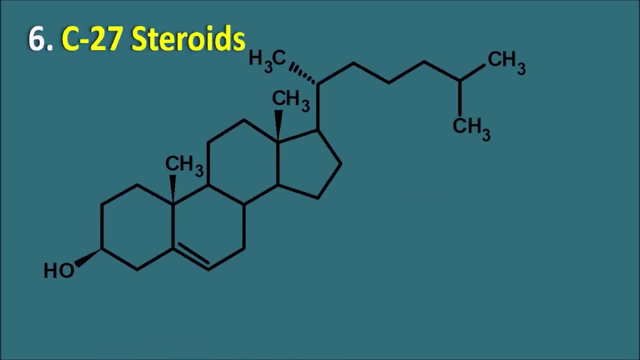 next one is the c27 steroids. so this is the c27 steroid and and the name of the nucleus is the cholistin. so this is one of the lipid that is present in the plasma membrane. this is the cholesterol, and in this cholesterol we can observe the oh group. at the second position, it can be: and the cholesterol isましょう. when you take a cholesterol taken, it can be taken by capsule in the very same way as the cholest aluminum. as the sch? слыш might be taken ab? utor f? primero o microlov S? for the choline ne? jail. in this case, where there is sounds that water meets scrapped, it gives. 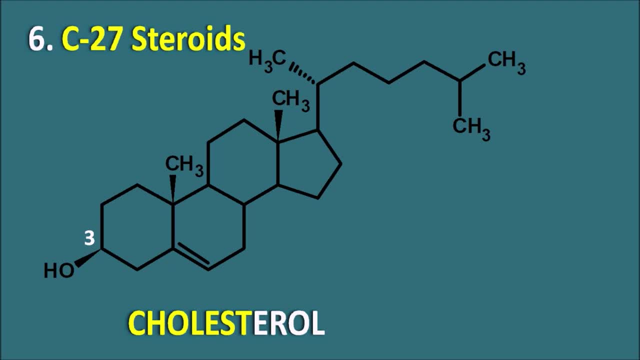 so the choline 20 mean it have products, muo cического is from separate and this is the cholesterol we shears. at the third position, which is attached by beta linkage, and it is having a double bond at the fifth position in the androgens and the progesterones. the double bond is present at the 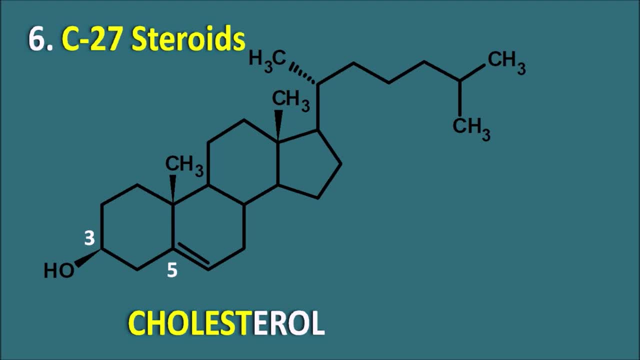 fourth position. but in the cholesterol it is present at the fifth position. so this is the cholesterol. so it can be written as colist 5 in 3 beta all. so it's having the double bond at the fifth position and oh group at the third position. cholesterol is one of the important lipid in the 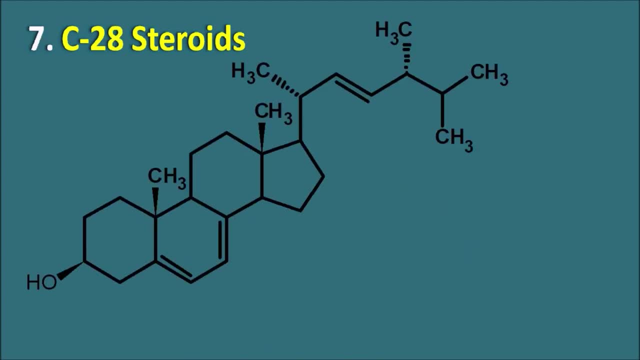 mammalian cells, but in the fungal cells, and the lipid is present. that is a ergosterol. so this ergosterol is a c28 steroid. that means it's not a c27. cholesterol is c27, but it goes there. on c28 you can observe an extra ch3 group at this side chain. that's why it is having the c28 nucleus. 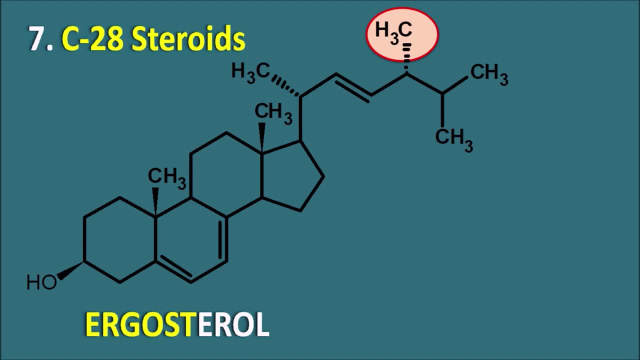 and the name of the nucleus is the ergostain which is modified at the different portions. third portion: it is having the oh group, just like cholesterol, and fifth portion is having the double bond. but apart from this it is having another double bond at the seventh position as well as at the 22nd position. so ergosterol can. 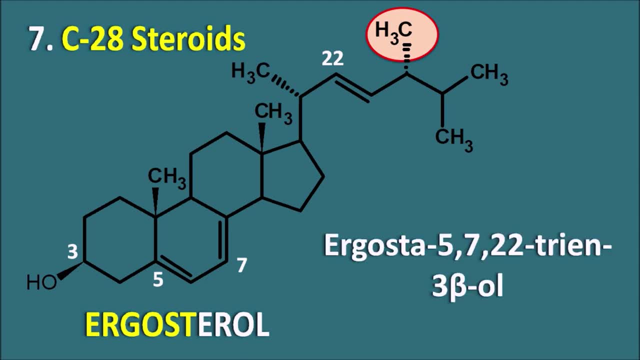 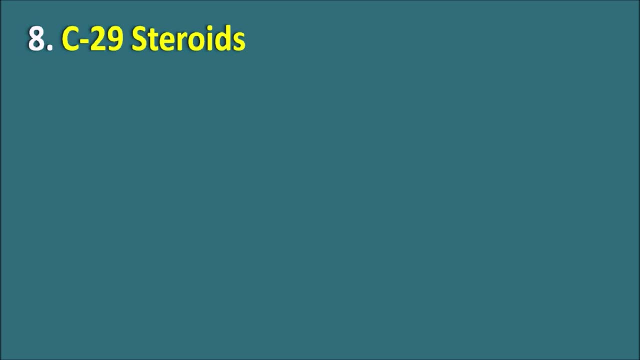 be written as it is a ergosta 5722 triene 3 beta old, so that is the ergosterol. next one is the c29 steroids. in the plants we can observe the c29 steroids, so this is a stigmasterol, stigmasterol. 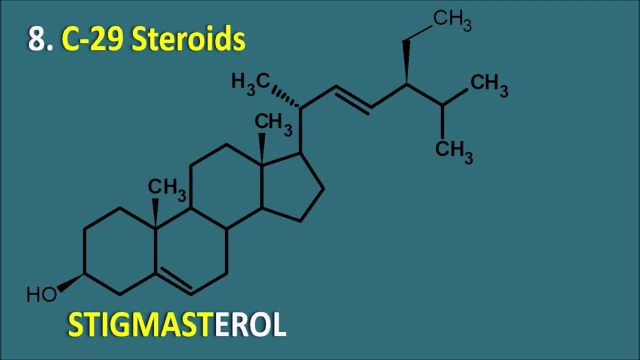 is having the stigmastern nucleus which is having the 29 carbon sterodial ring, and here you can observe that at the 24th position it is having the two carbon ethyl site chain. so 27 plus 2 it becomes 29, and again it is in the third portion, oh group, attached by beta linkage. 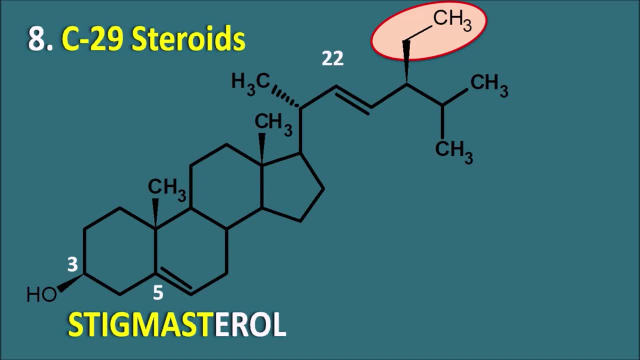 fifth portion, a double bond is present and 22nd portion, and the double bond is present. so stigmasterol is the stigmaster 522 diene 3 beta wall. so this but licke sterol is having a nucellular nucleus which is having the 29 carbon sterol ring, and here you can observe that at the 24th 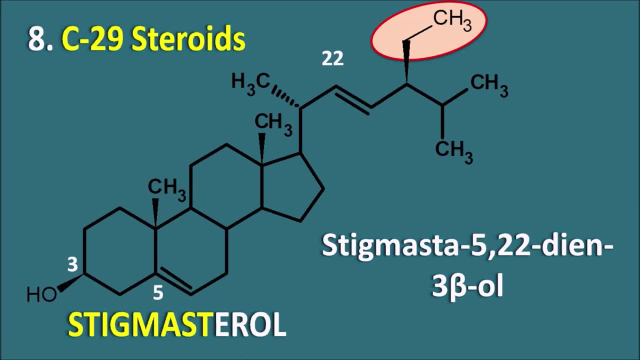 This stigma sterile is present in the plants as a lipid. 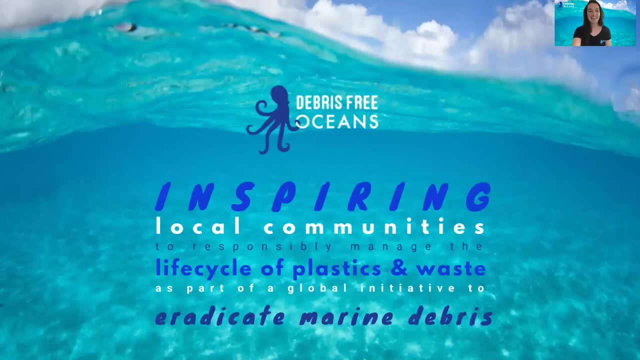 Hi everyone. Thank you guys so much for having me today. My name is Maddie Kaufman and I am the program director at Debris-Free Oceans. We are a 501c3 nonprofit based out of Miami and this year is our mission statement inspiring local communities to responsibly manage. 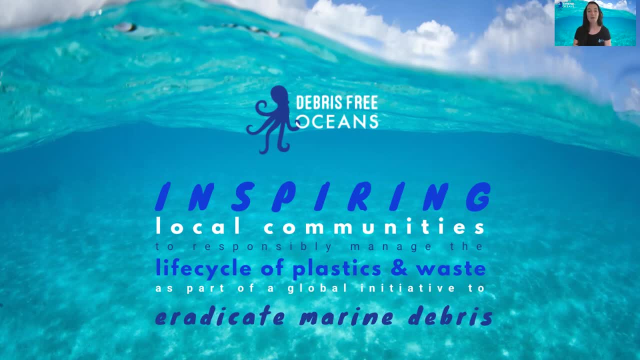 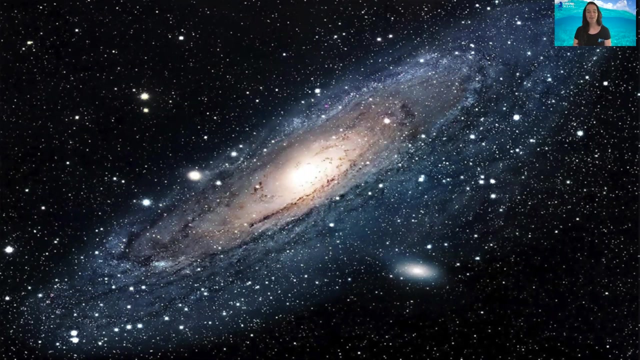 the life cycle of plastics and of waste as part of a global initiative to eradicate marine debris. So I'm going to talk to you guys about why this is so important and how you guys can get involved, So to give you guys just a scale of the problem and start a little bit big picture.